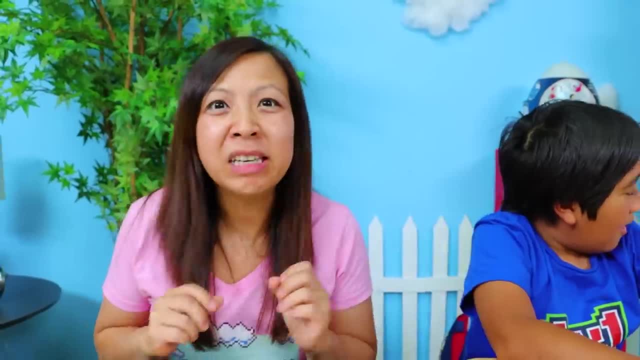 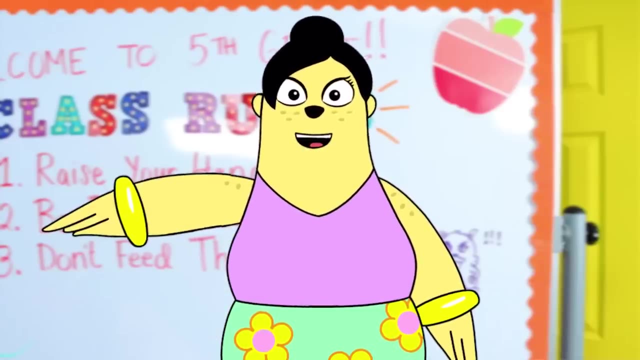 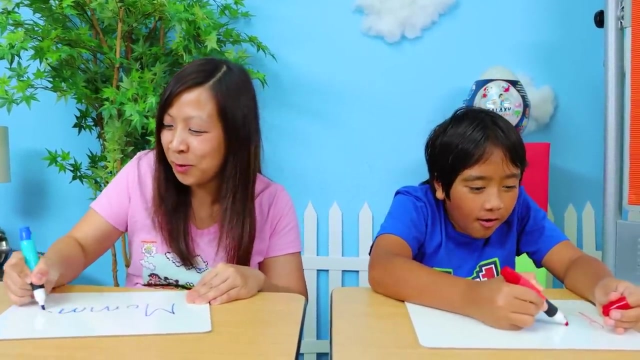 Hello, I am right here. Seems a little scary, don't you think? All right guys, Now for your first assignment. go ahead and write your name on the board in front of you. Easy, Fifth grade is going to be so easy. Definitely know my own name. My name is Ryan. 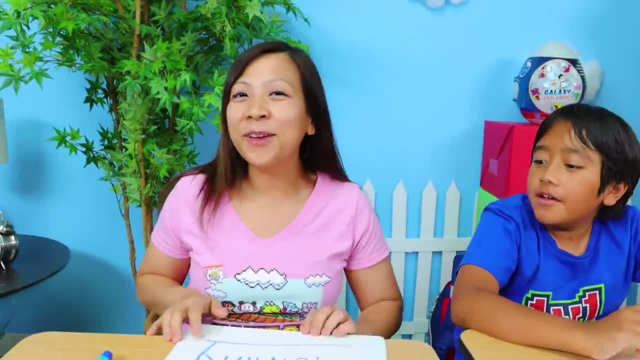 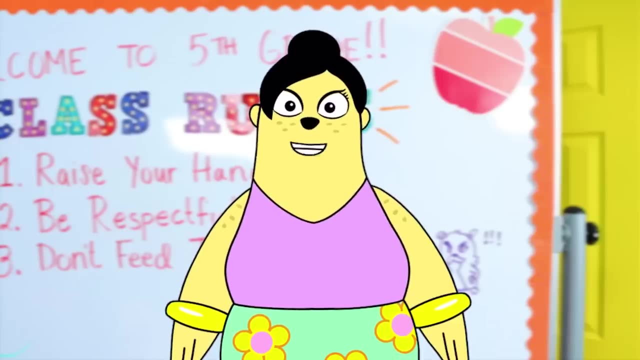 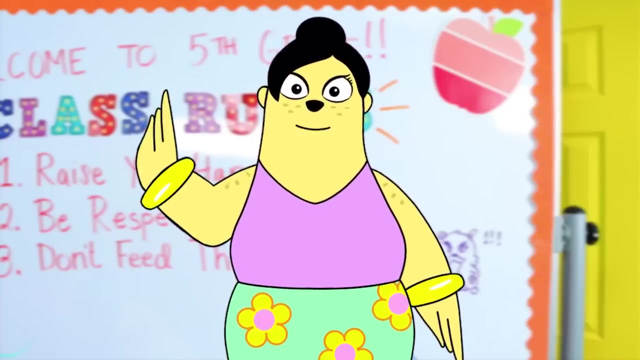 Hi Ryan, Thank you for coming in, And my name is Mommy. Oh, welcome, Mommy. Well, are you guys ready for your first class of the day? Yes, All right, Your first teacher is Mr Drew for art Here. he is Easy, I love art. 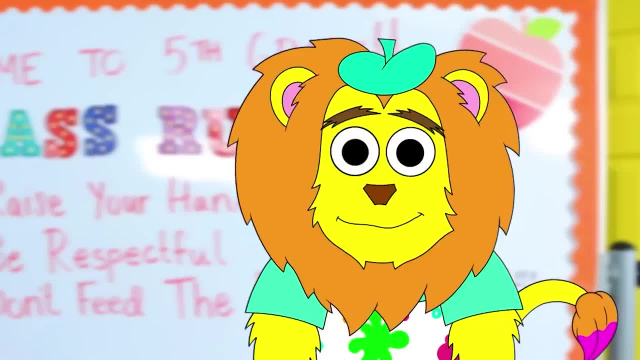 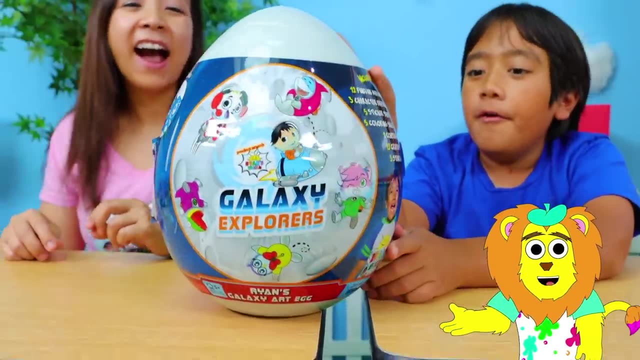 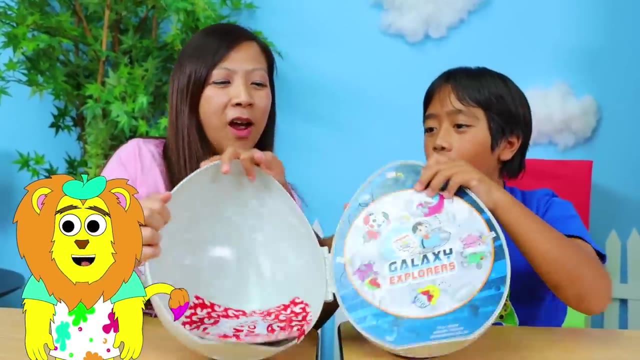 Hi everybody, Welcome to art class. Are you guys ready? Yeah, In front of you you have the Ryan's Galaxy art egg For your first assignment. I want you guys to open it and create an artwork that reminds you of all the fun you had during. 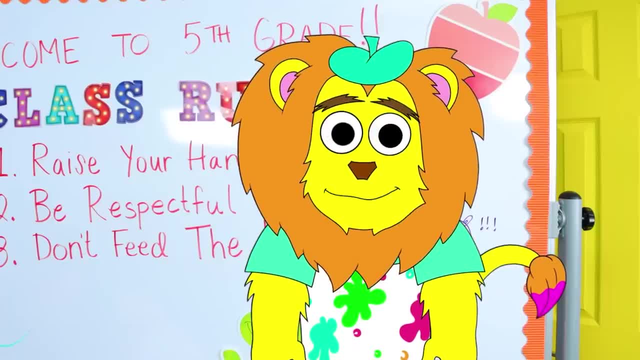 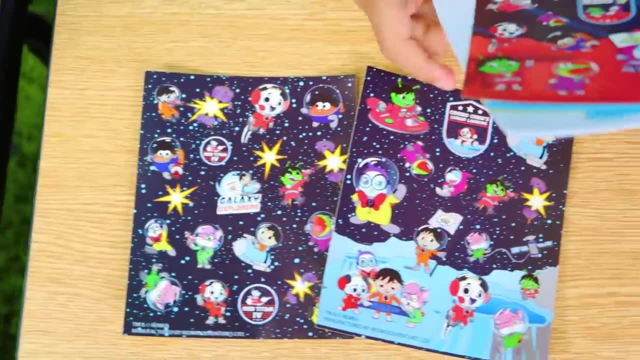 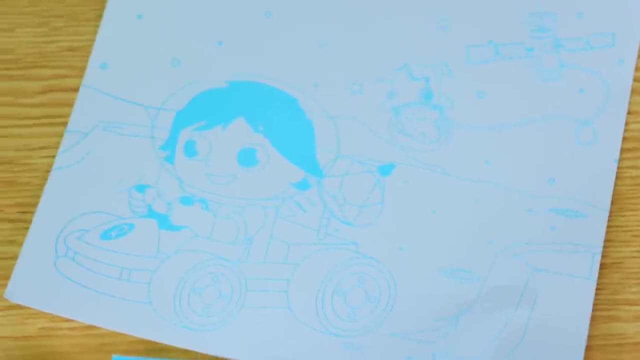 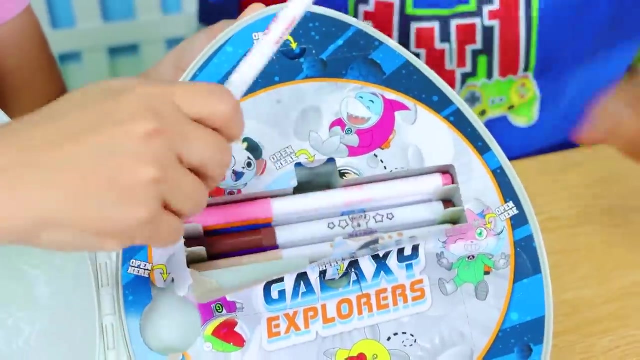 the summer. All right, have at it. I'm excited to see your artwork. Oh, there's some stickers. Galaxy Explore theme- Yeah, I like it. And there's some peaches to color in. What else is inside this Galaxy Explore egg? Oh, eraser and some markers- Oh, I'm not going to love the little. 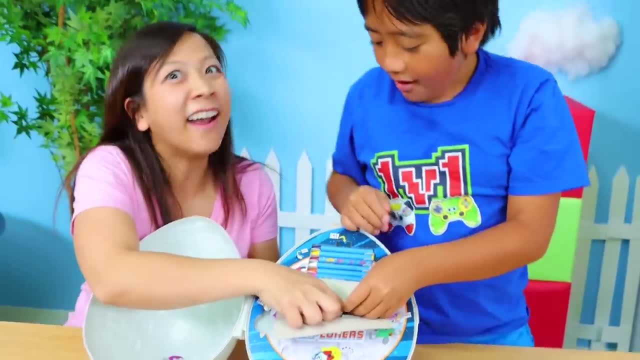 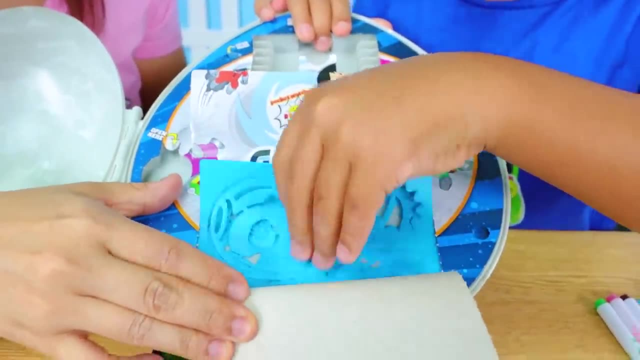 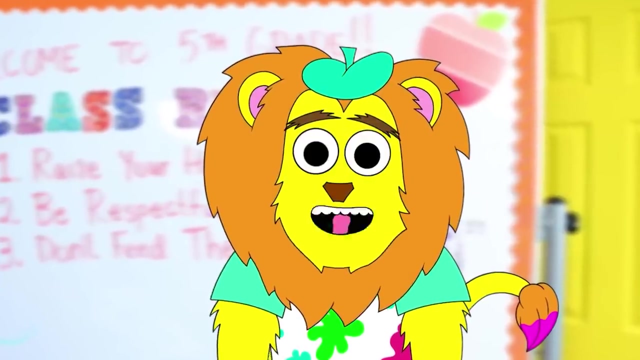 pictures there. It's like a mo Crayon. Yeah, I'm going to need this for sure. Some stencils Cute. All right, Ryan, you ready to get started? Yeah, Now you will have one minute to create. 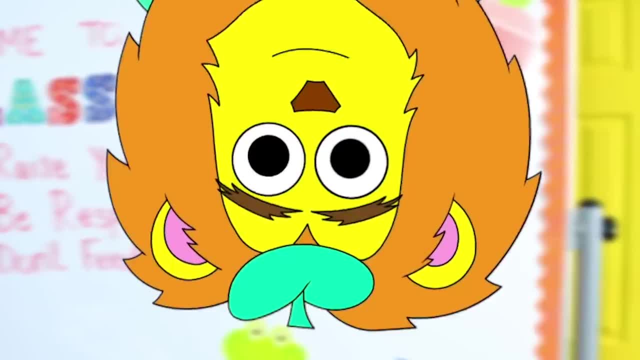 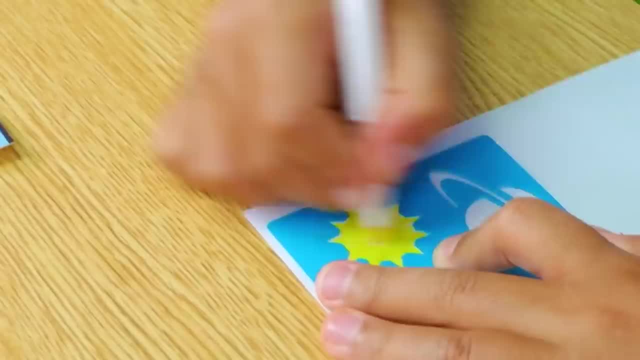 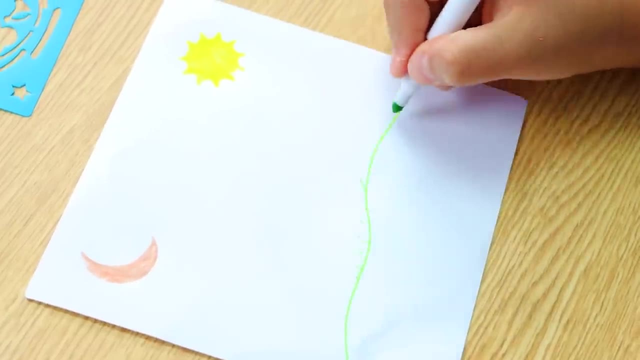 some awesome artwork. Three, two, one go My best art in one minute. that's it Got to color it in. Art class is hard in fifth grade, but I'm doing such a good job, right guys? Okay, I'm drawing some land right now. I don't have enough time to color it in, so I just got. 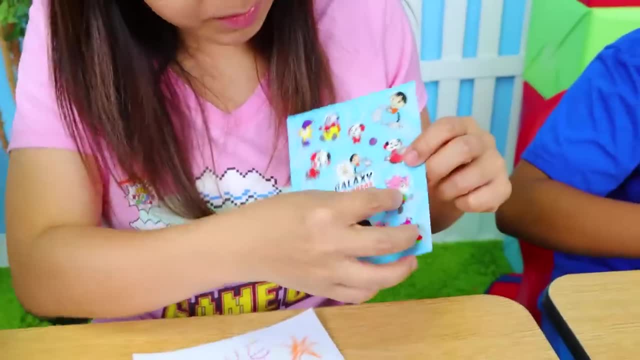 to put some grass. okay, Almost done. All I'm going to do is add some stickers I'm going to have. I'm going to teach Alpha Lexa, of course, Floating in space Next to love I'm going to put. 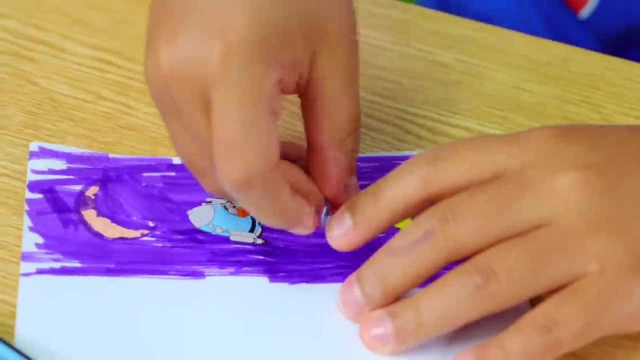 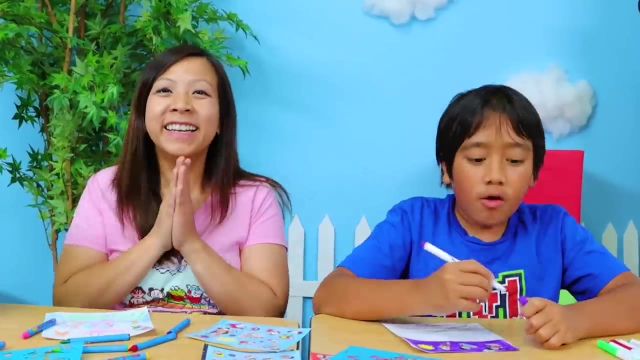 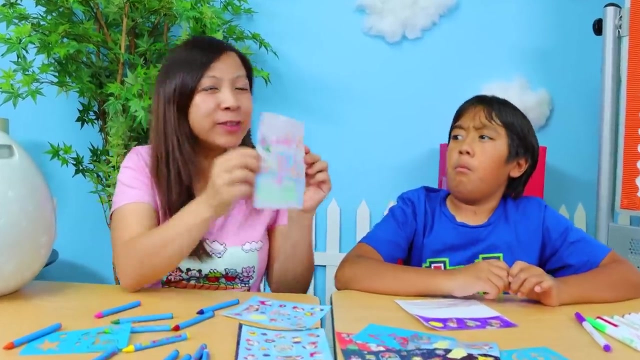 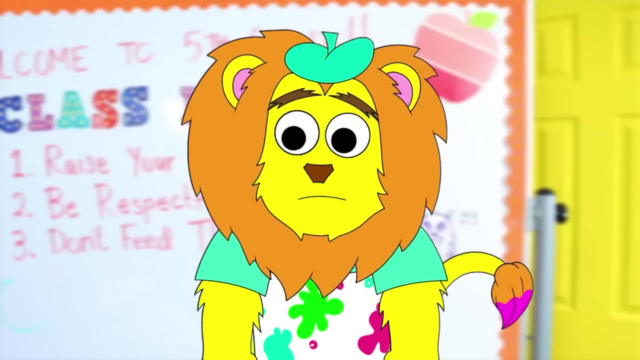 myself flying in space with my friend Combo Panda. Okay, time's up. My favorite part: Let's show off your art. Okay, Mr Drew, this is my artwork here. right, I even put the cute little touch that says love. Hmm, Uh-huh, You did pretty good, but Combo isn't that. 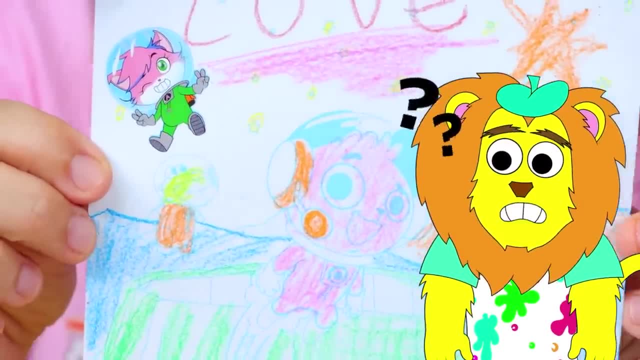 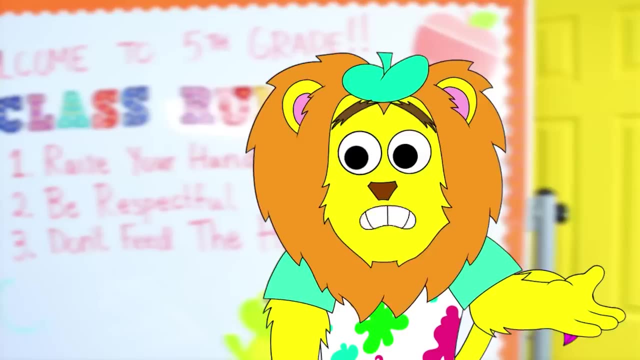 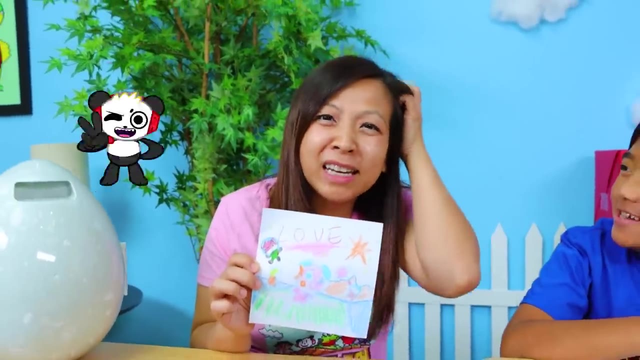 color? Um, he looks like he's very warm and red and his headphones aren't even the appropriate Red. Going to have to give you a B, A, B. Wait, what color is Combo's headphone? again Red, Oh, I forgot. Okay, Ryan, let's look at your artwork. 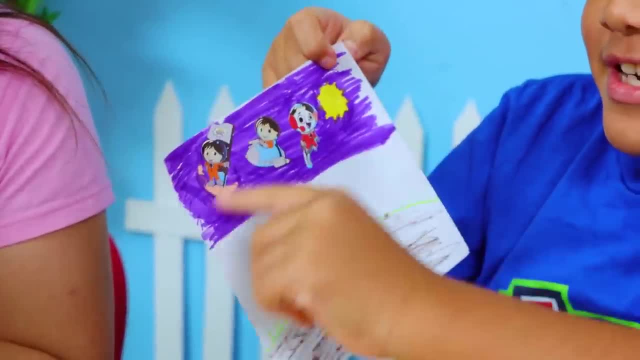 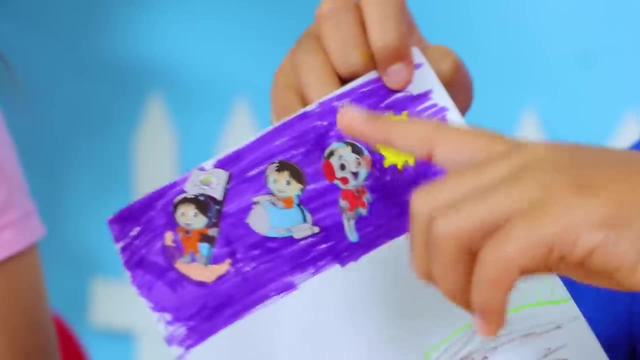 So there's the land, here's the sky. I drew the sun and the moon, and it's nighttime. Uh, I was so powerful that I duplicated myself to be the first one on the moon. and uh, I'm also flying. 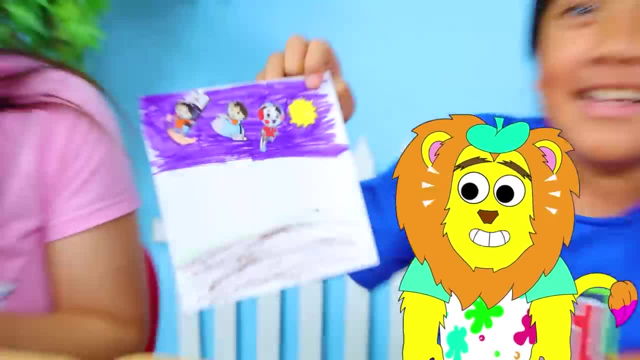 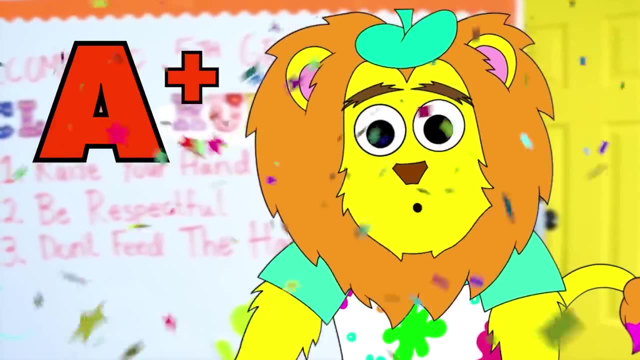 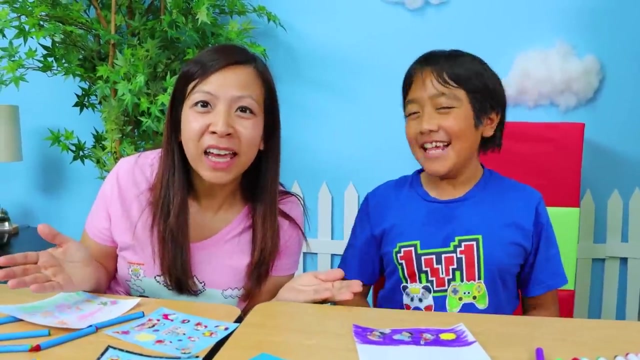 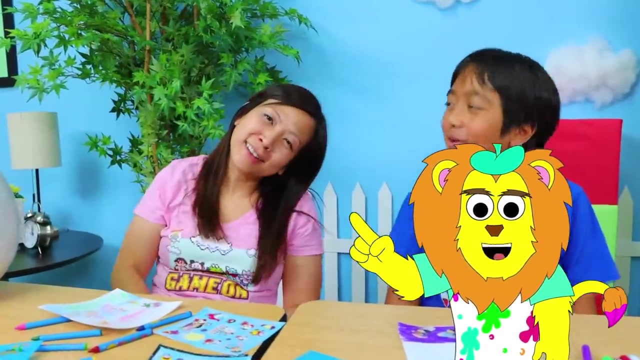 Flying to my duplicated self. Wow, The creativity on display is just it's breathtaking. I think I'm going to give you an A++. Wait, yeah, Is that even a real letter? grade A++. He duplicated himself, so I duplicated the plus every time. Well, excellent work, class, Great first day of school. 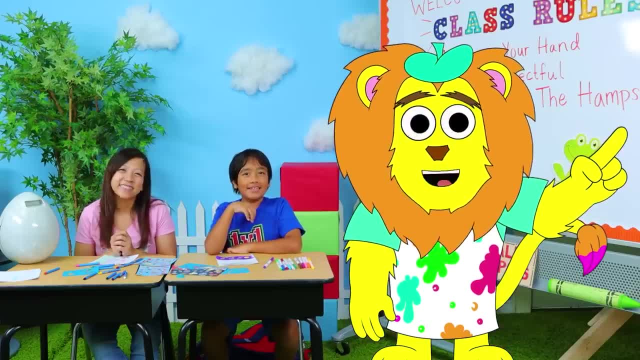 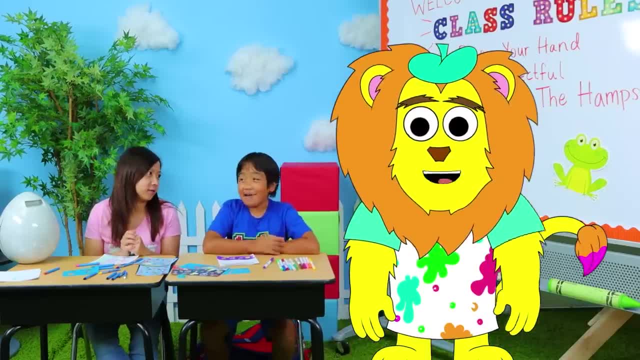 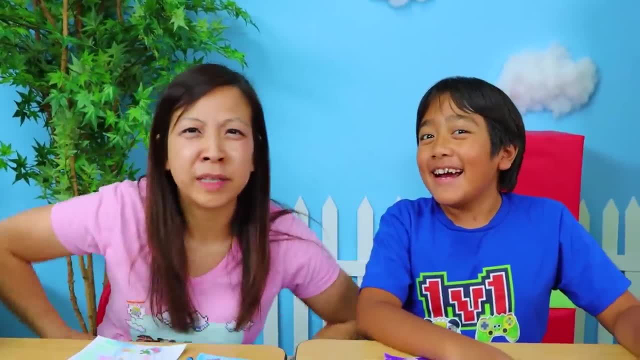 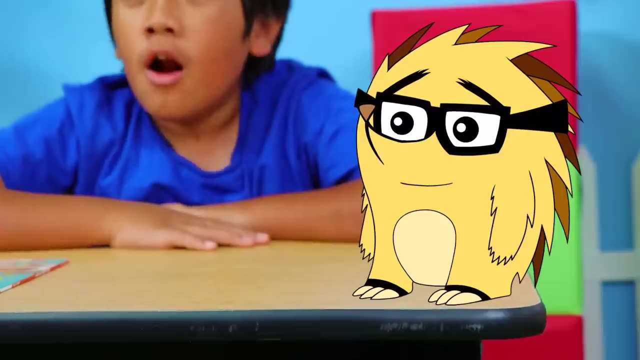 But anyways, bye, everybody. Your next teacher is coming over now. Bye, No, I hope it's science. I am so good at science and I'm better. Where's our next teacher? I'm right here, guys. Welcome to science class. I'm Mr Zoomy. Thanks for coming today. Are you ready for your first experiment? 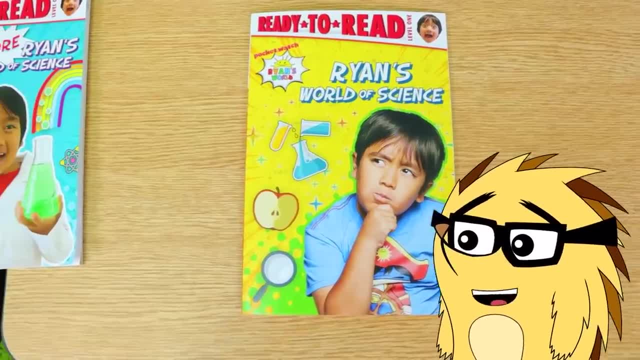 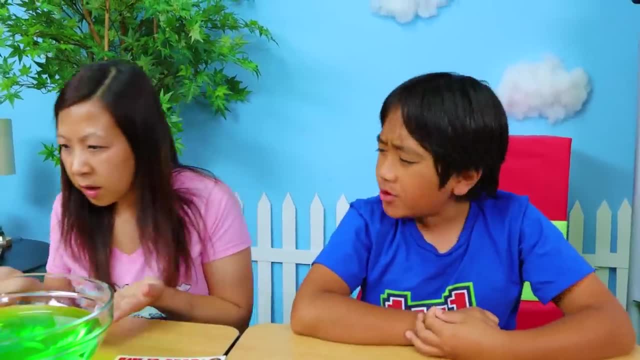 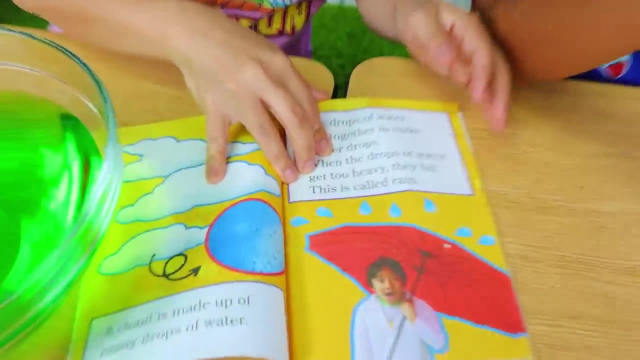 Yes, Yes, Let's get started. Your reading materials is on your desk. Go to the science books to find an experiment for today. With the materials that we have, which science experiment would work? Okay, we have something with water and some objects. Let's see here. Oh, I don't think so, Is it? No, I don't think this one. Oh, not the s'mores experiment, We don't have that. 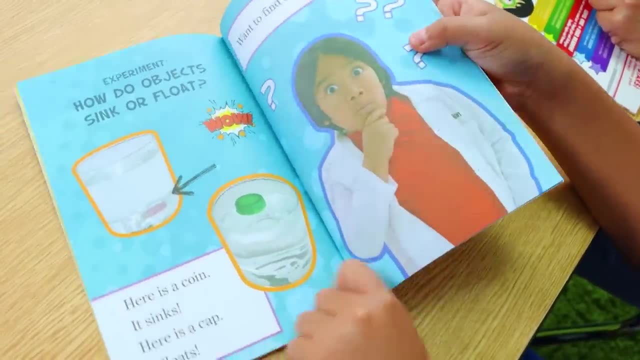 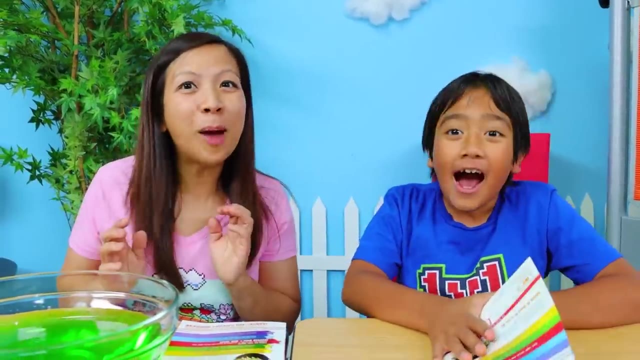 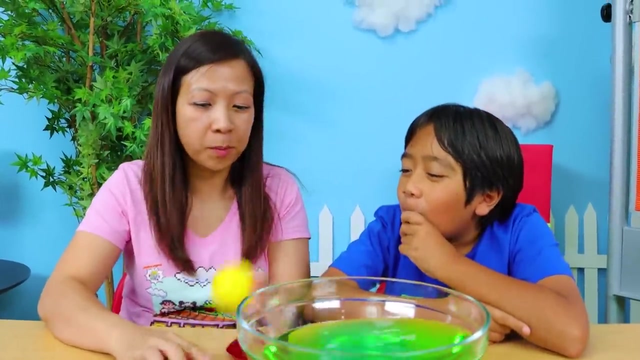 How do objects sink or float? Here is a coin: It sinks. Here is a coin cap- it float. maybe that's our experiment. good job, ryan. so we have to figure out if these objects are float. are you ready? oh, what is your hypothesis? what about this ball float? uh, okay, i think it. 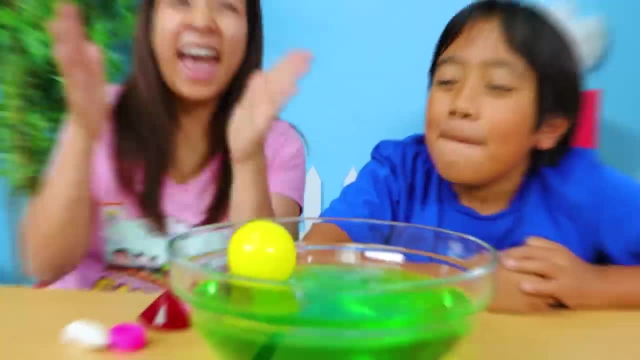 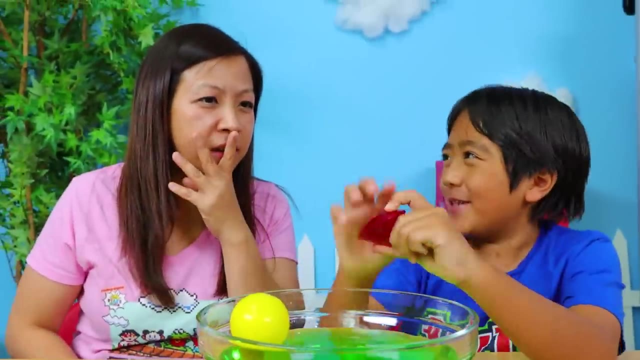 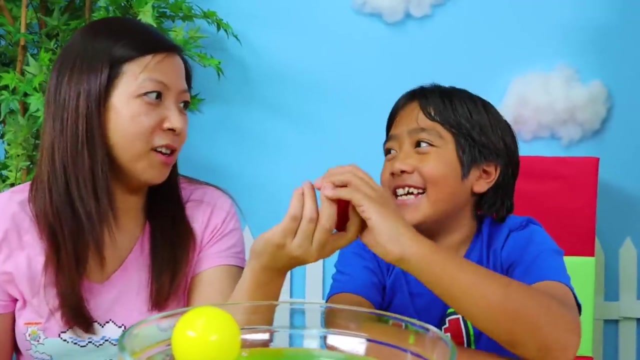 floats too. i should know this. let's see. yay, okay, you ready to do next gym? okay, gym. i think. what's your hypothesis? you go first. this gym is not real. it is a fake gym, so it's going to float. i think it's gonna sink, are you sure? yeah, okay, let's see. oh, no, it's pink. yeah, okay, you know what? 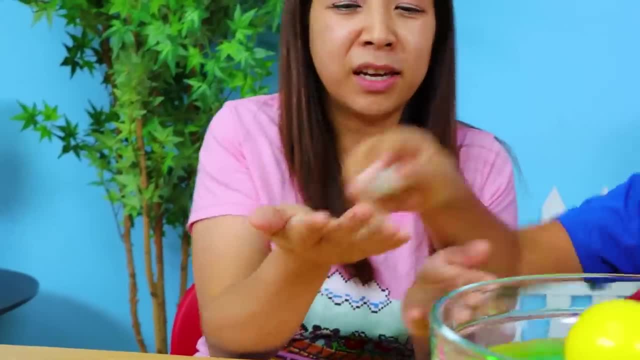 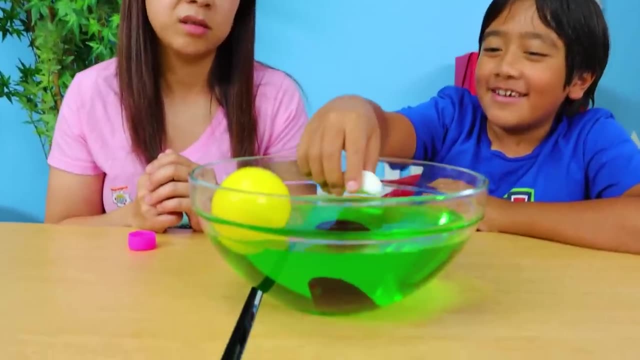 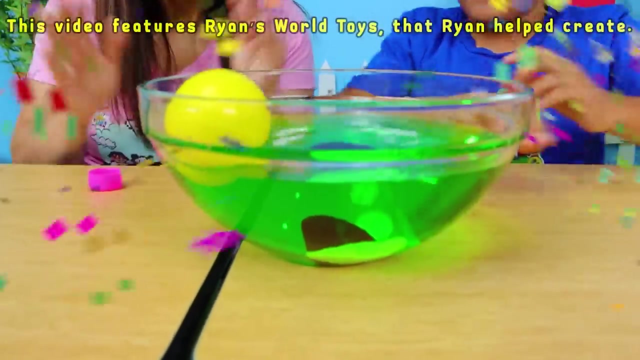 it's not over. it's not over. okay, what about this rock here? let me feel it. okay, hover, are you sure i think it's safe? rock six: oh, it's hovering, have to drop it. yay see, i told you i'm good at science, okay, last one is a bottle cap. oh, in the. 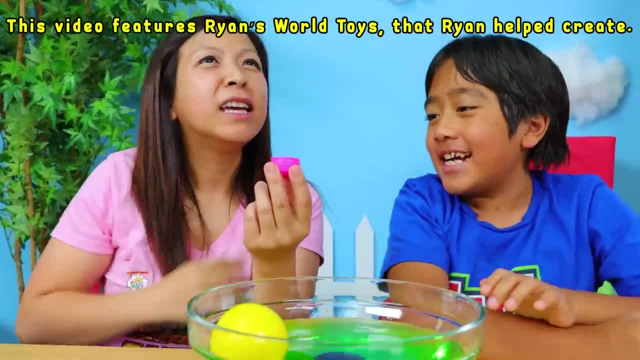 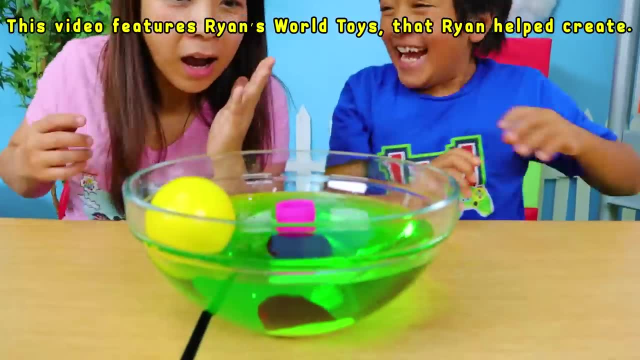 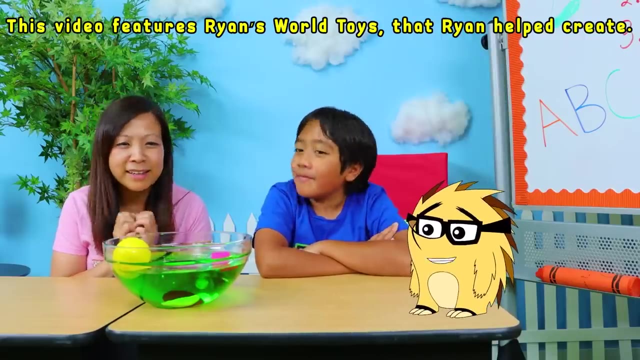 book, i forgot it said it. it sinks actually. oh, and the books are the same. yeah, it might be a special bottle cap. yeah, got it okay. sinks then. yeah, floats. oh no, i wonder where my grade is gonna be. all right class. excellent job hypothesizing the results. i think i'll give you some grades before. 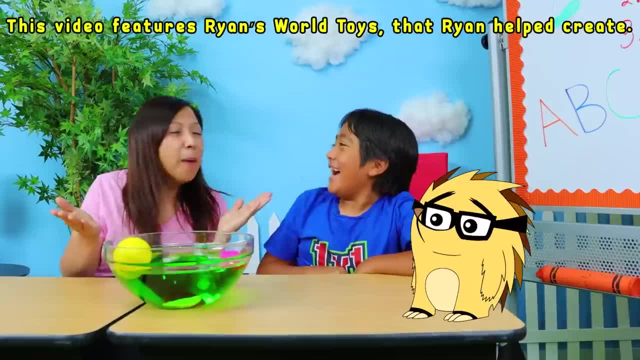 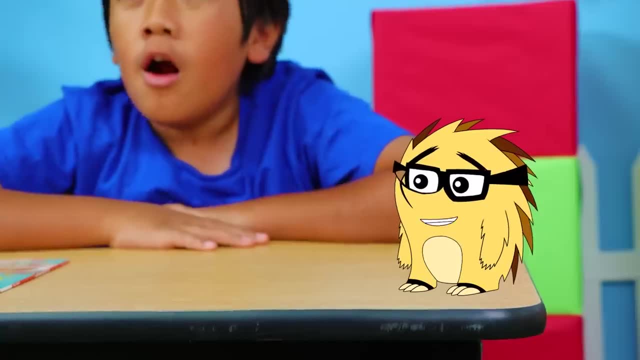 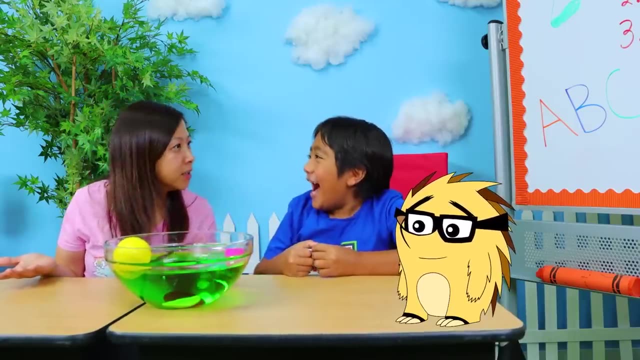 we go on to our next lesson. mommy, you're going to get a, b, a, b again. what about ryan? what do i get? i think i'm going to give you a different kind of grade. i'm going to give you an s plus. s is better than a. what does it even mean? s plus, he gets a special. 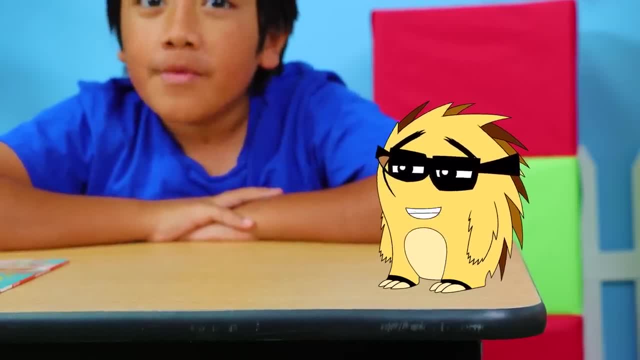 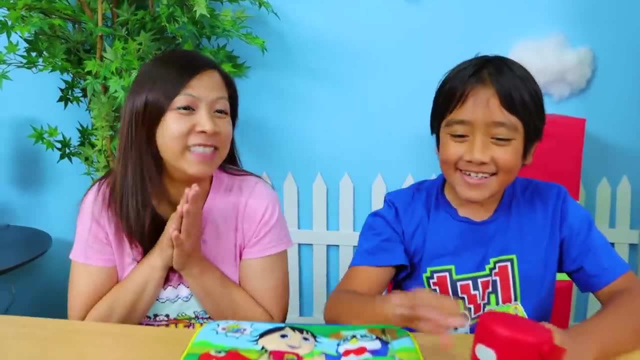 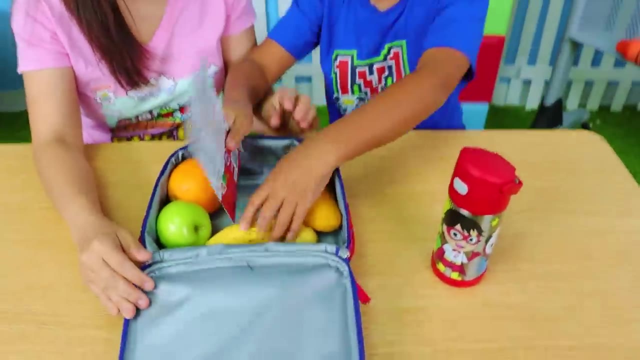 bonus for reading the right experiment and not just getting through the pages. good job, ryan. yeah, all right, it's time, snack time. i love snack time. what did we bring again? i forgot what i packed. i don't know, of course. okay, so we got some yummy fruit and the thicker you can eat. 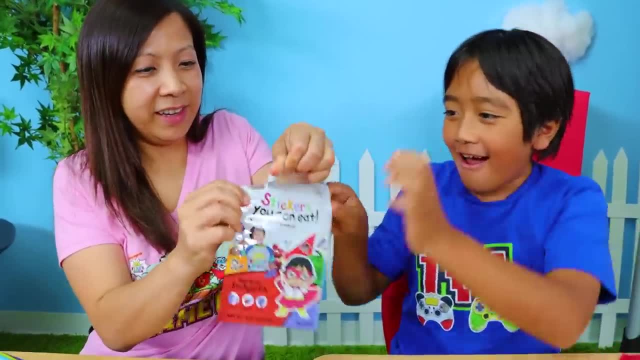 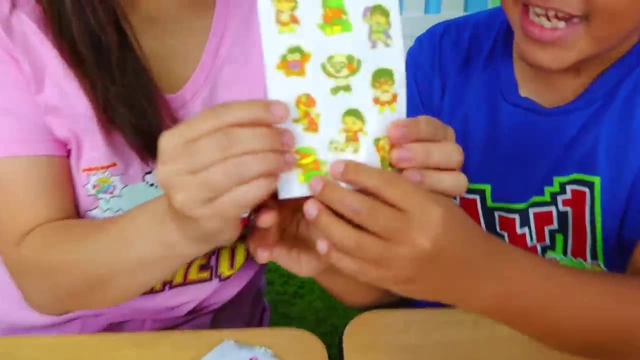 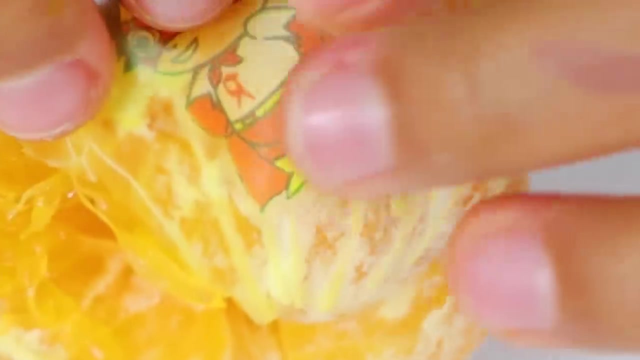 what stickers you can eat. i want to try, okay, okay, and even have ryan's world characters on it. so, look, you can just eat them. yeah, then you put your stickers on a piece of fruit or vegetables. my turn. okay, here we go. all right, bye-bye, combo. 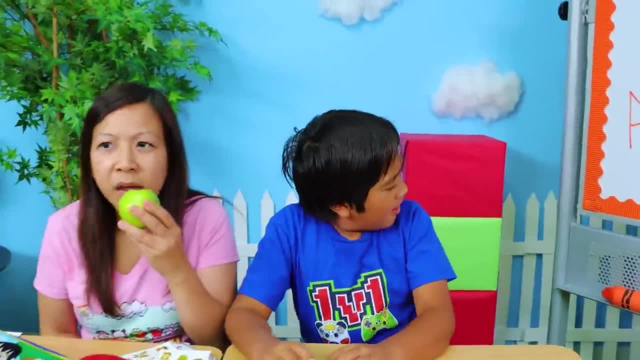 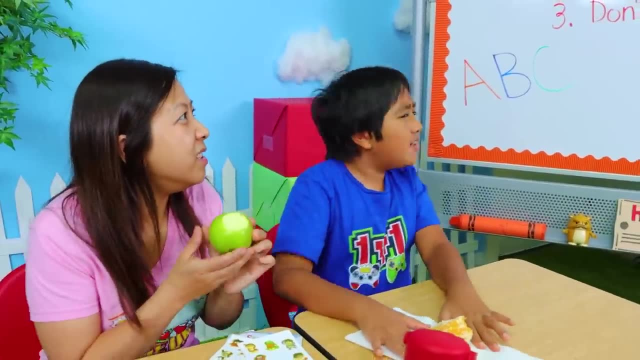 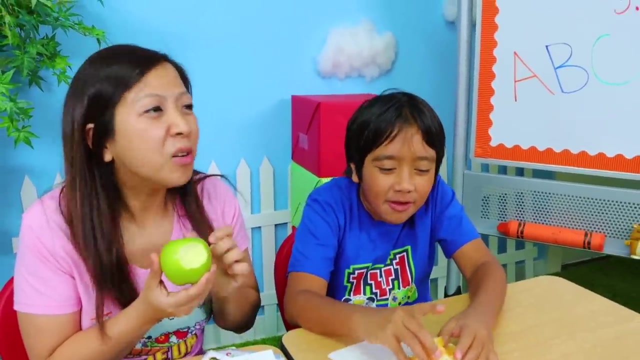 are you guys gonna finish that? who's that? oh, um, i don't, i mean. i mean i i guess i could share with you, but it says: don't feed the hamster, it's fine. nobody's here, are you sure? one time more, okay, yeah, he looks pretty hungry. 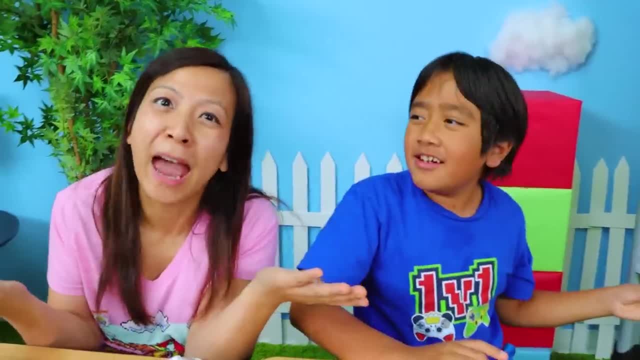 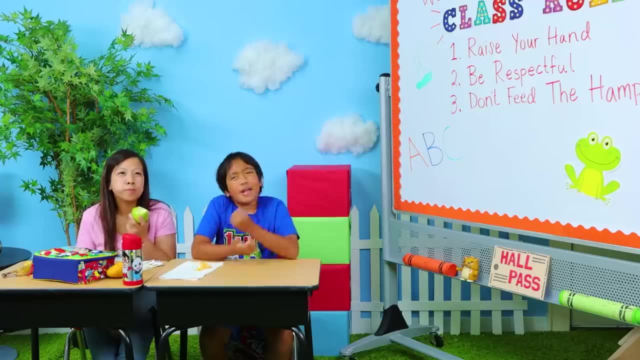 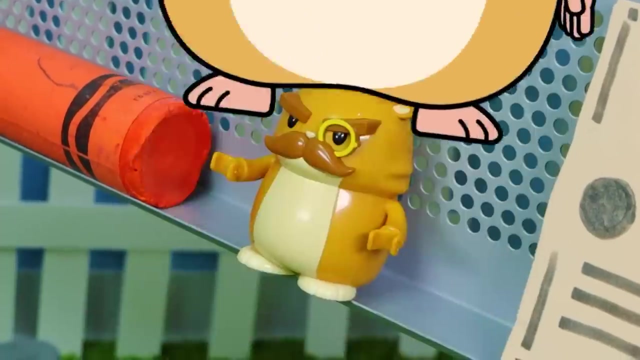 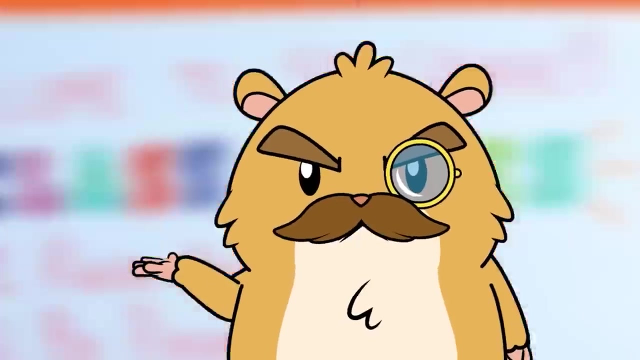 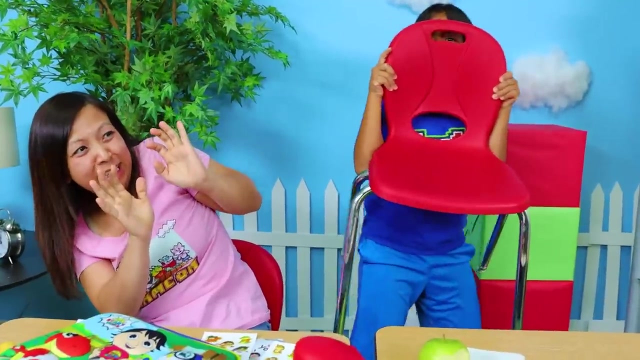 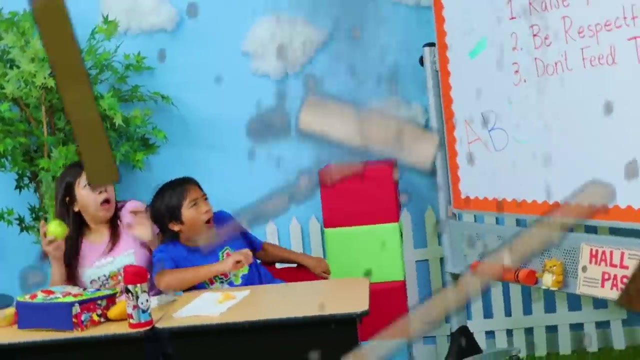 okay, all right, ryan, you go wait. what's the worst that could happen, am i right? he looks super cute? yeah, yum yum yum. sharing is caring, right? yeah, what's the worst that could happen? yeah, thanks a lot, guys. now i am catch this little Connection, little Connection. 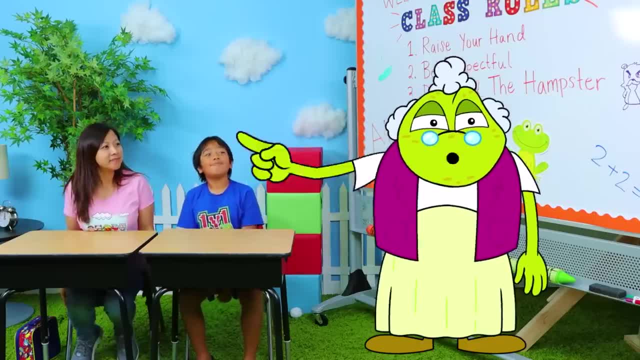 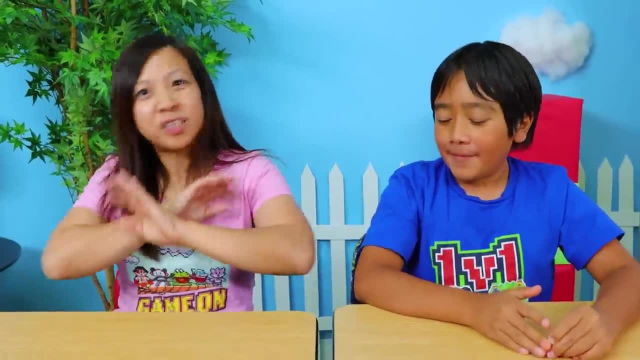 all right, i need to go do some evil hamster deeds. see you all later. oh no, do we actually do something wrong? next teacher's coming abnormal. i'm okay, hi everybody. a? Oh no, we cleaned up and everything looks pretty normal, Am I right? 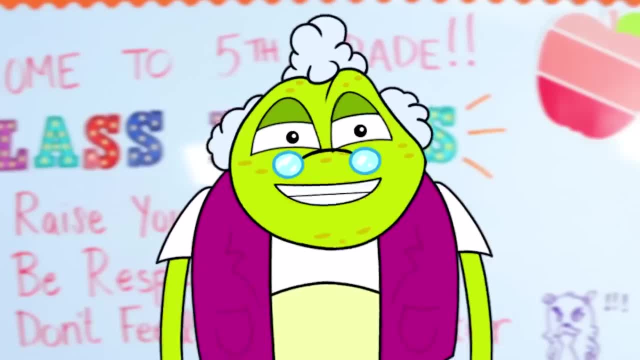 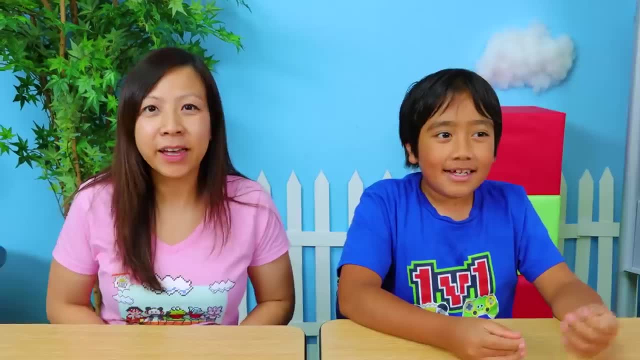 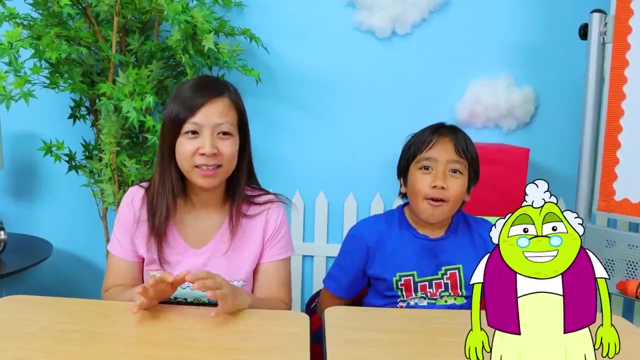 If you say so, I'm your math teacher, Ms Lilypad. Today we're running through some equations, but since it's your first day, we'll start off easy: Two plus two, Two plus two, two plus two. I remember it was five. 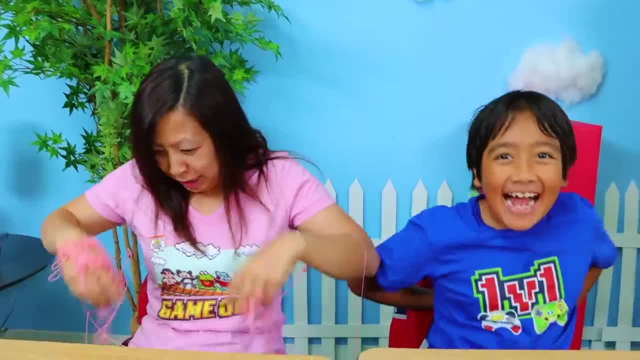 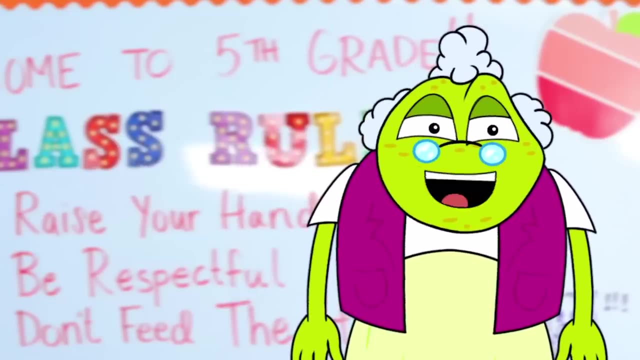 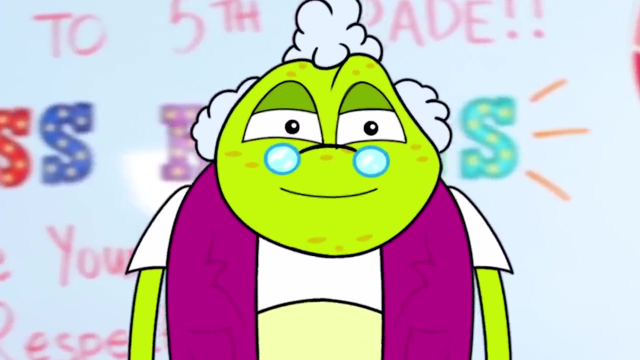 It's five Five Four. That came out of nowhere. Where'd it even come from? I told you you should have studied your math during the summer, Sorry, the next question. I got it this time, Okay. Next one is eight times eight. 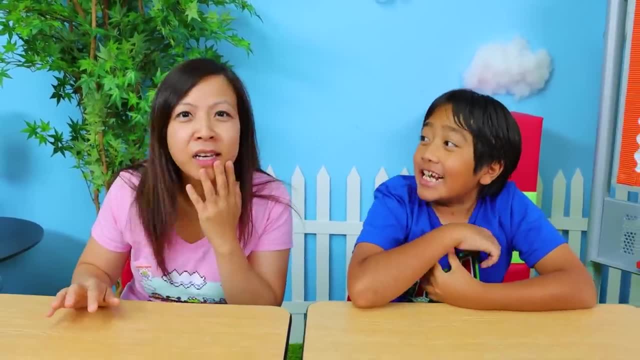 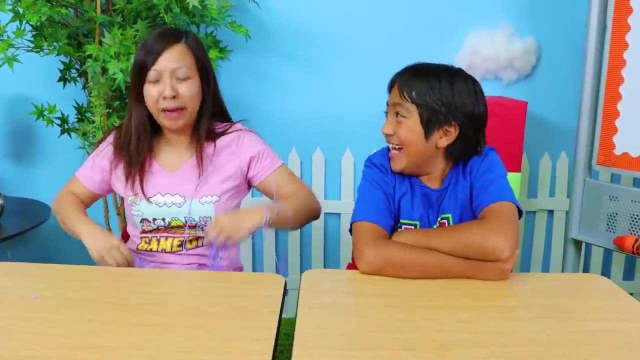 Eight times eight, eight. wait, what did she say? Eight plus eight, Yeah, eight plus eight, Easy 16.. Okay, okay, I really should have paid attention and studied in the summertime. Okay, but next one, I totally got it. 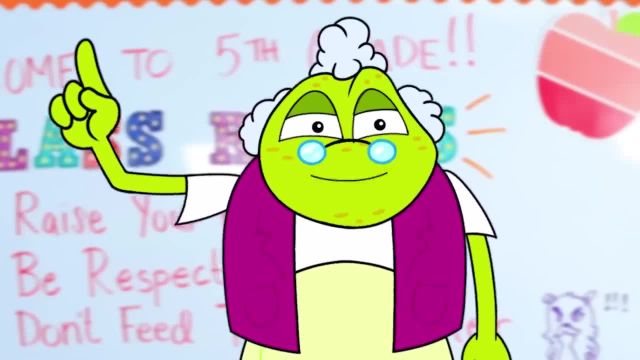 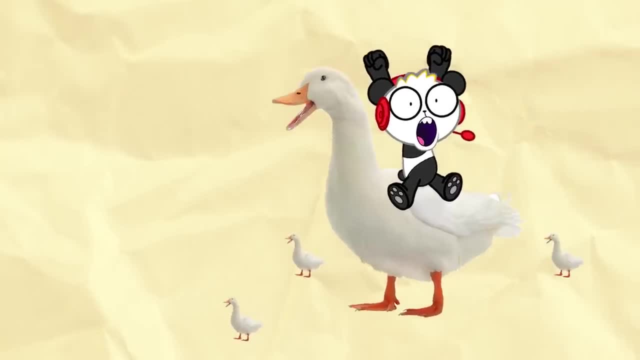 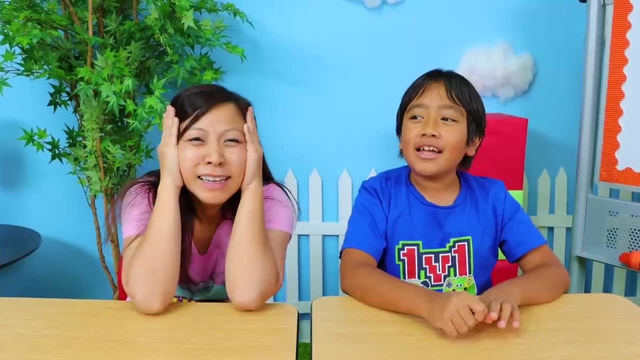 I got it this time, All right. next up is a word problem If Bob has four ducks and they're all crossing the road simultaneously and they bump into eight more ducks and then cross the road with a chicken at the same time. 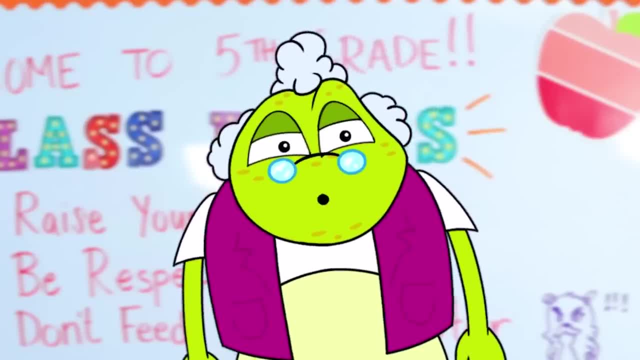 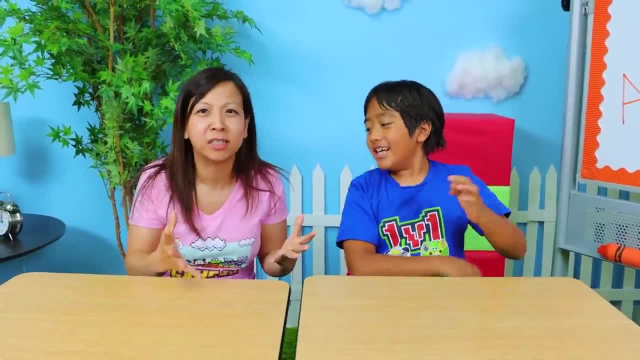 what are they going to find on the other side? Oh, it's fish. Wait, how, I don't know, it can't be. There's ducks, and then there's chickens. They're gonna see more ducks and chickens, am I right? 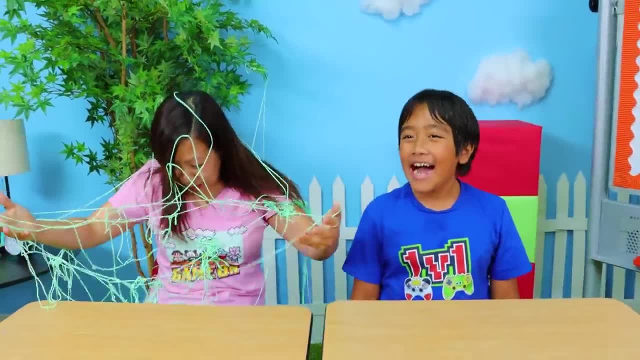 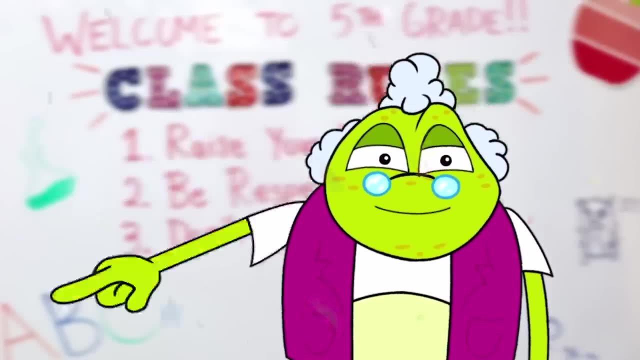 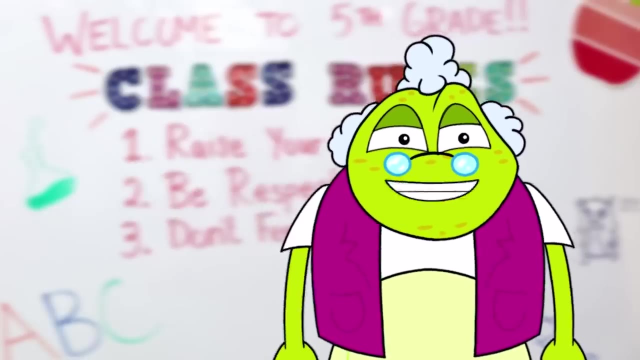 No wait, you couldn't make sense. The question doesn't even make sense. Ian, you get an A plus plus for all your hard work. Oh, no wait, does that mean I have to repeat this grade? Luan, you're gonna have to come in for tutoring, sorry. 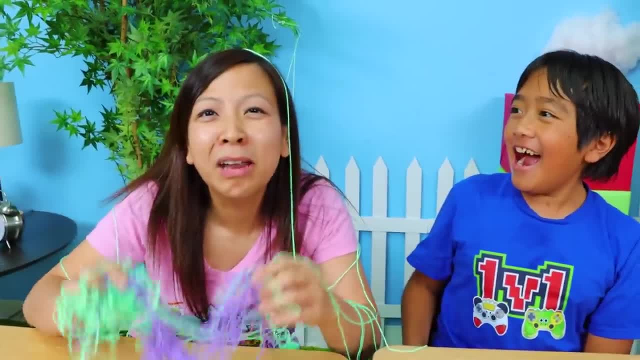 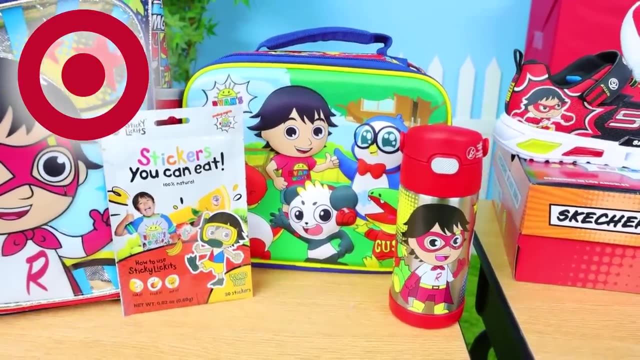 Oh yeah, also every day is bring your mom to school. then Oh no, The Ryan's World Mystery Art Egg is available at Walmart. The Ryan's World Lunch Bag with insulated compartment, double zippers and padded top handle is available at Target. 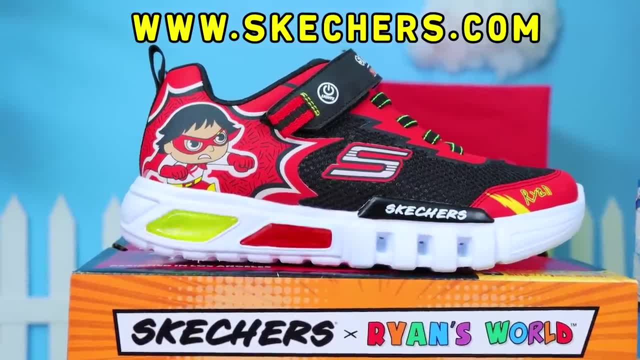 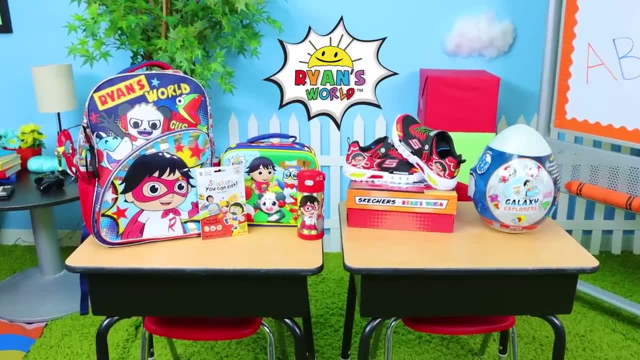 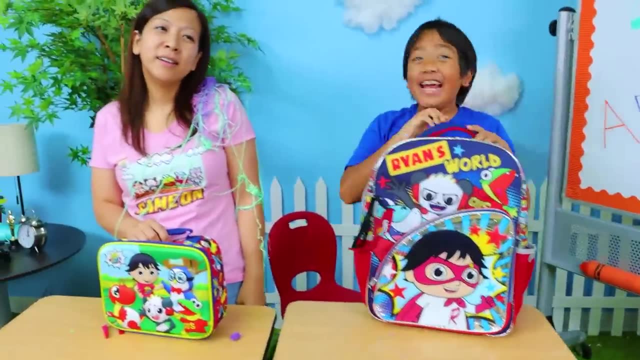 The Skechers Ryan's World Collection is available on Skecherscom. Parents, start your kid's new school year off on the right foot with Ryan's World back to school gear. Ryan's World has your back to school shopping needs covered. Okay, Mommy, I think you gotta start studying. 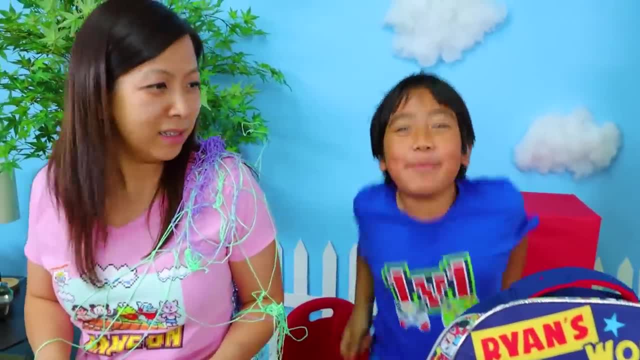 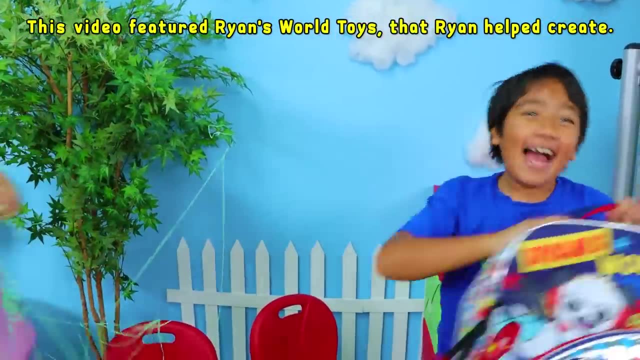 Bye, thank you. Thank you for watching. Remember: always: stay happy and rise up. Bye, All right, that was such a fun first day of school. Bye, bye, guys, Bye. This video featured Ryan's World toys that Ryan helped create.